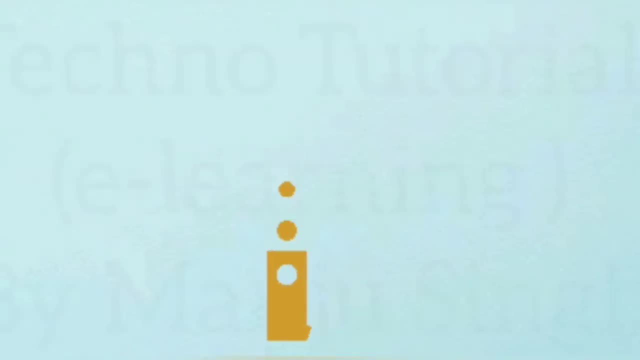 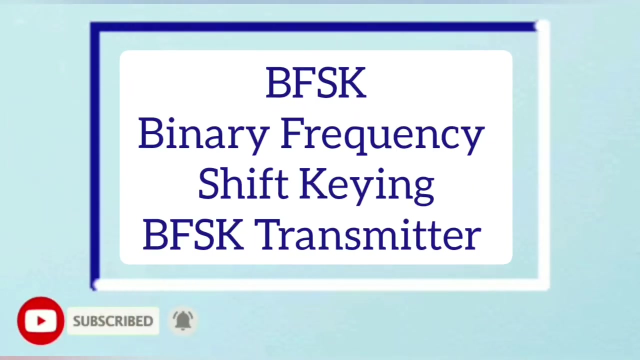 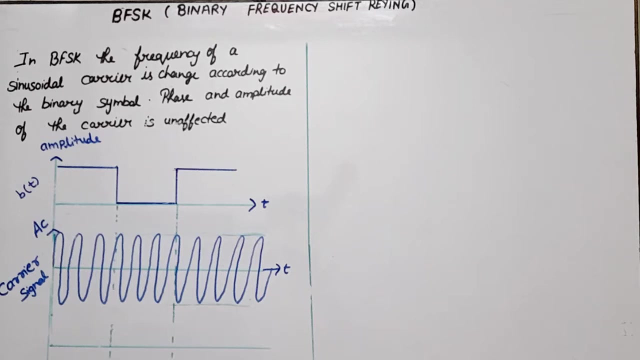 Hello everyone, in this video lecture of digital communication I am going to discuss BFSK. BFSK stands for Binary Frequency Shift King. As name suggests, this is frequency shift king means frequency of carrier signal will change according to the binary symbol or according to. 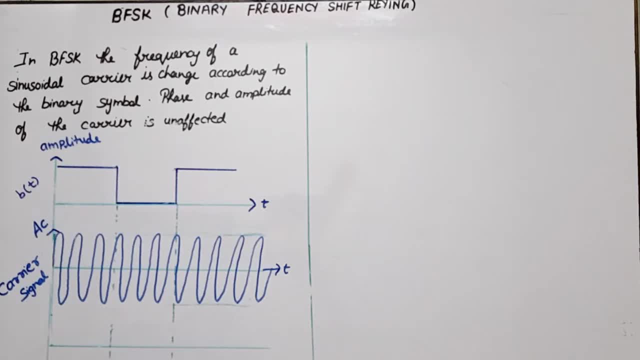 the bit stream. Now, in this case only frequency will change, hence phase and amplitude of carrier signal is unaffected. I have drawn two waveforms here. First for bit stream BT. this will be our unipolar signal: 1 0, 1.. I have taken only 3 bits. 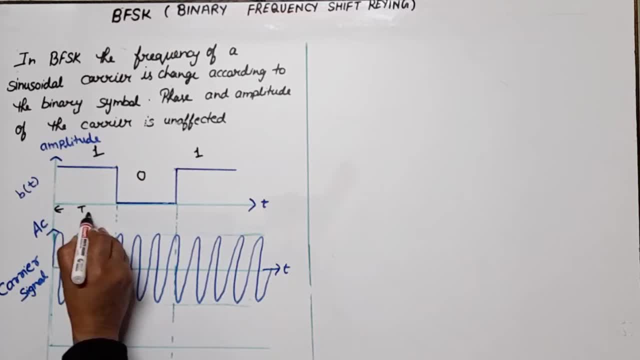 And this is the bit duration: TB Clear Bit duration. This is our carrier signal whose characteristic changes, So in this case its frequency will change. If your bit 1 will be transmitted, then frequency will be dense. If bit 0 will be transmitted, then frequency will be rare. 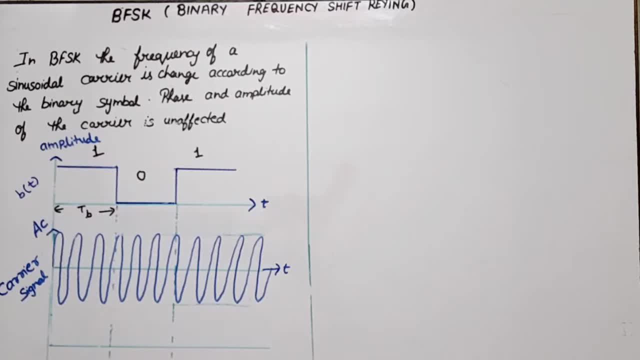 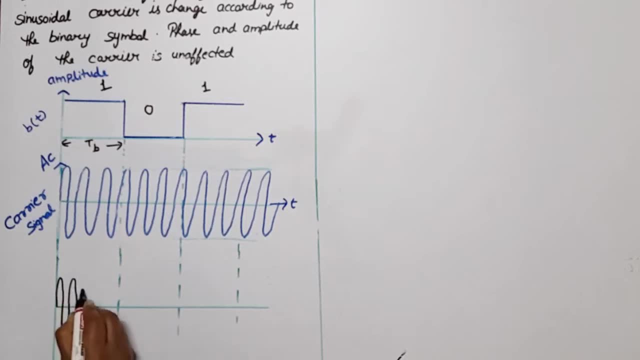 means it will be less in comparison to actual frequency. Now let's see Bit 1. frequency will be dense Bits 10.. If I will transfer bit 9, this frequency will be more. Number of cycles increase: here it was 3 and here is more than three. Now bits 0 for symbol. 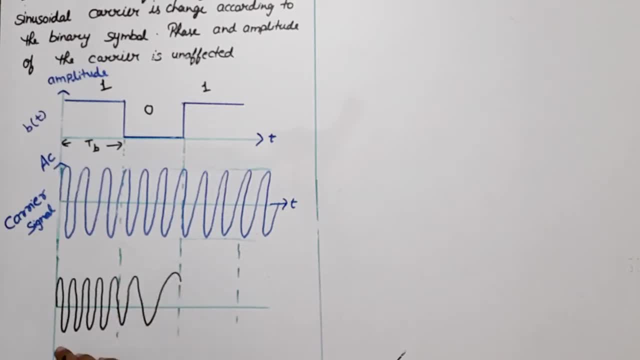 0 or bits 0. Number of cycles was more in actual, but here it is less, Again 1. Alright, So what we got? 4. When vit 1 is transmitted, then we will get 4. 4. 4.. 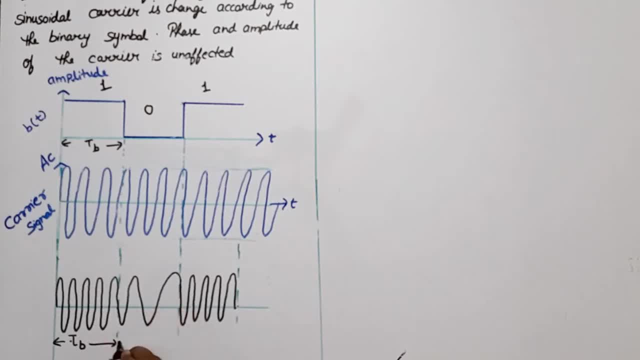 4. 4.. meet hoti hai frequency high. when bit 0 transmit hoti hai, for that bit duration, frequency will be low. yeh hamara, kya hai actually hamara? yeh hai ac amplitude mein no change. and this is b f s k signal. now yeh hamara signal hogaya. according to this waveform, there is two frequency. 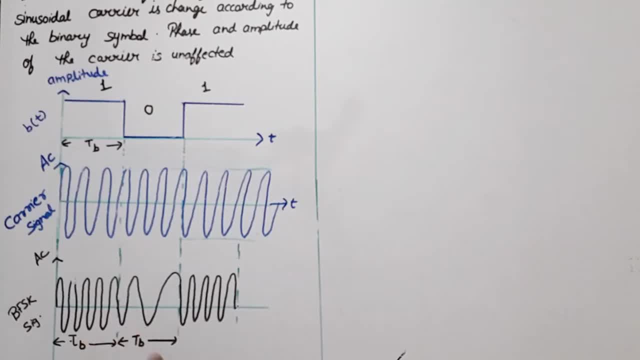 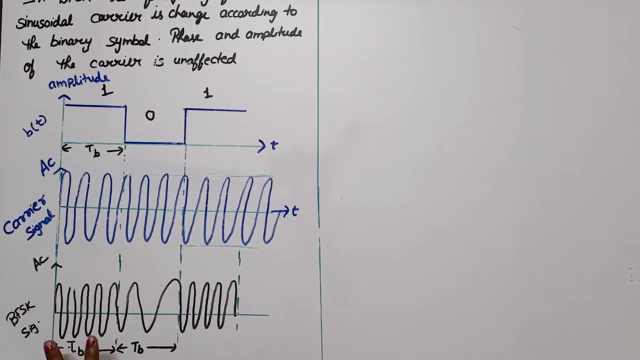 component: one for high frequency, one for low frequency. now ab iski equation likte hai. according to the modulated waves, mein ham kya use karenge two different frequency: one for one, that is high frequency, one for zero, that is low frequency. theek to now frequency, hence frequency symbol. 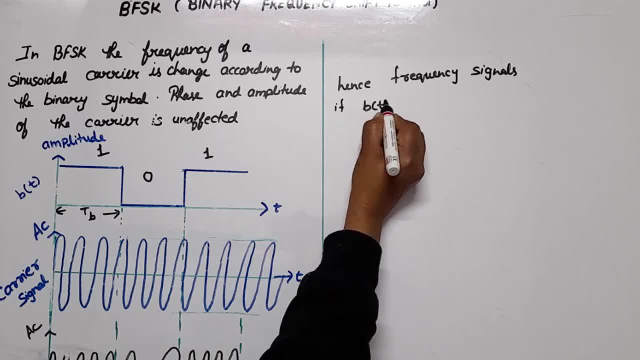 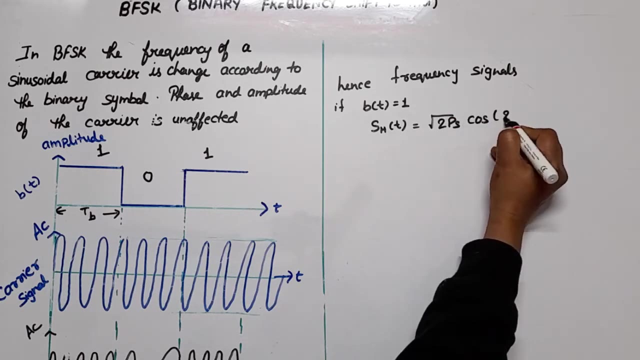 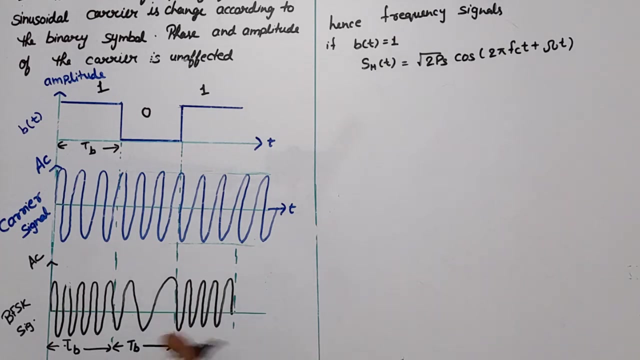 hence if b, t means ki if bit symbol is one, then kya hoga? ham isko mention karenge as h, t theek hai, because high frequency mil lagi thi. yeh kya hoga? hamara under root 2 ps, cos, 2, pi, f, c, t plus ohm fix amount ka increase hoga or fix amount se yeh decrease hoga aur. 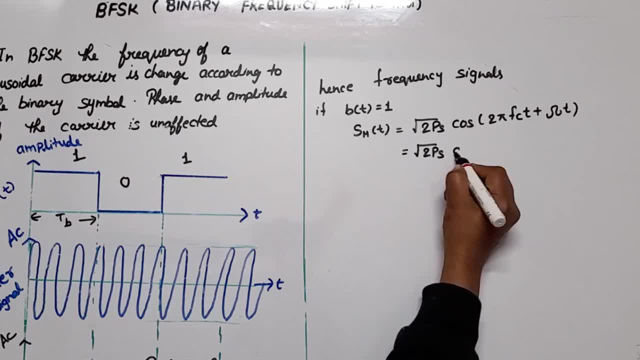 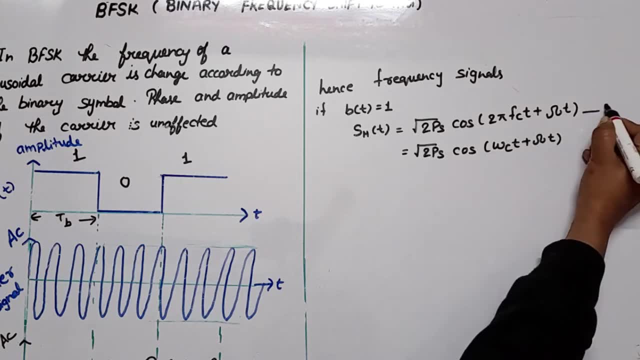 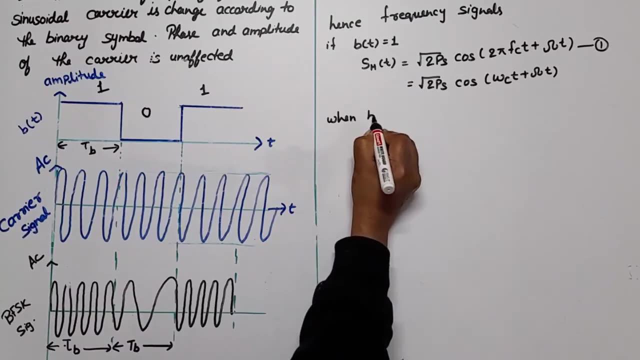 we can write it under root: 2 ps cos, omega ct plus ohm t. theek hai yeh hamari equation. one hogay now ab hamara. jab low frequency signal hai means when bt kya hoga, haise meerkat hai ok is equal to 0.. If bit 0 transmits, we have named the signal SLT, because frequency will be low under. 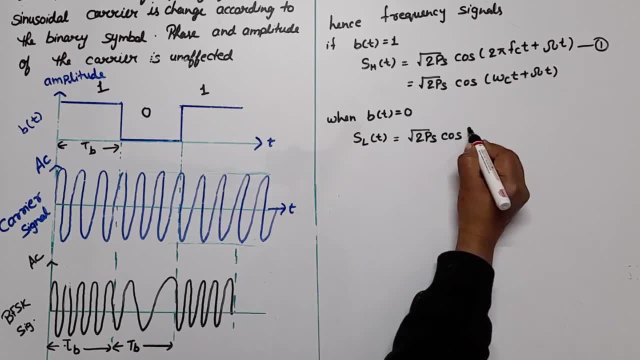 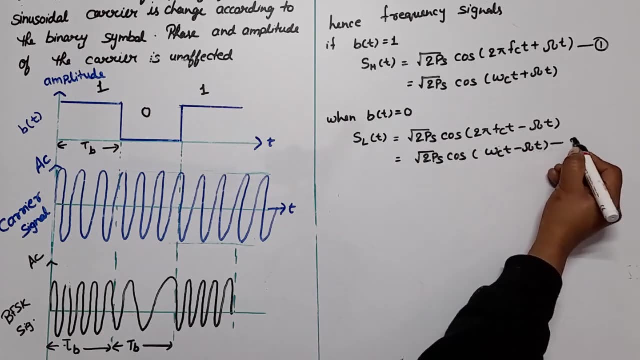 root 2 PS cos 2 pi FCT minus ohm T. Now it can be written as under root 2 PS cos omega CT minus ohm T. This is our equation number 2.. Now, if we combine these two, then what is the equation? 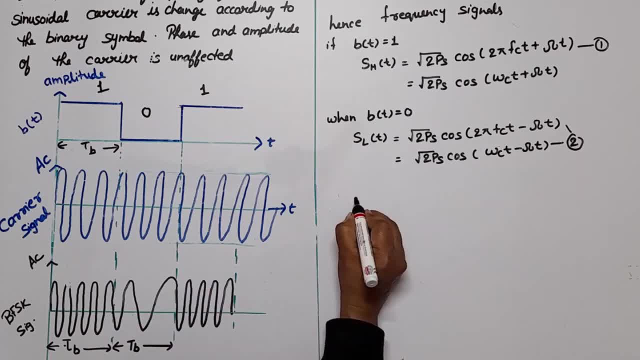 which will be our actual Combining 1 and 0, what will be the equation? finally, BPSK is equal to under root 2 PS. What will be the equation? Either plus or minus? what can we write? Cos 2, pi, FCT. 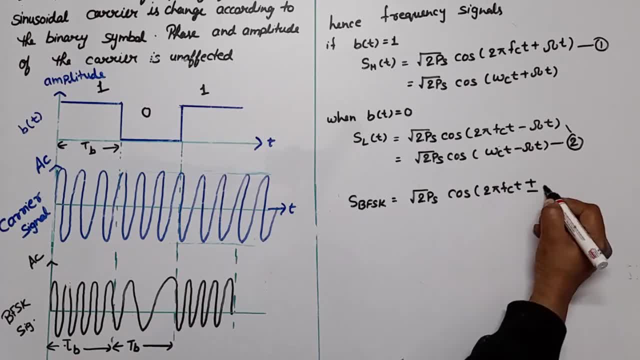 plus in case of 1, minus in case of 0 ohm T And under root 2 PS, cos, omega, CT plus minus ohm T. So this is the final expression for BPSK. Voltage label. representation of BPSK. 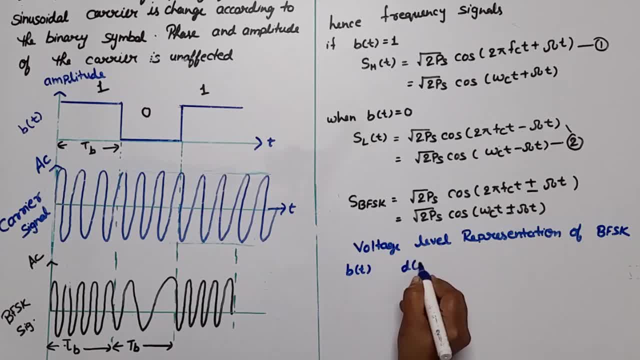 What will happen in this Bit? BT, then sign means plus or minus, then power for high signal and PLT for 0. If bit is 1, positive sign will be this one. So what will happen here? Plus 1 volt. 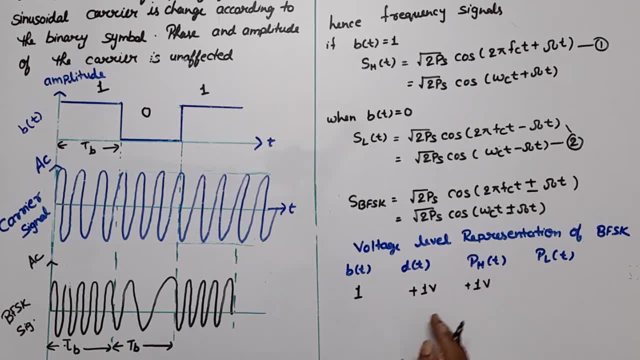 PH will be 1 volt plus positive. What will be the value of low 0.. Same way, if bit is 0, what will be the value of DT? Minus sign Means minus 1 volt. PH will be 0.. What will be the value of PL Plus 1 volt? 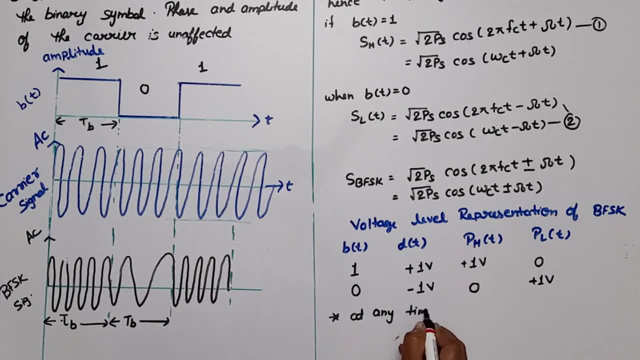 Any time, at any time, either PH or PL is 1. But not both In one time. only one will be on, Either PH or PL. Okay, We will use this, This. So what is this? This is the equation. 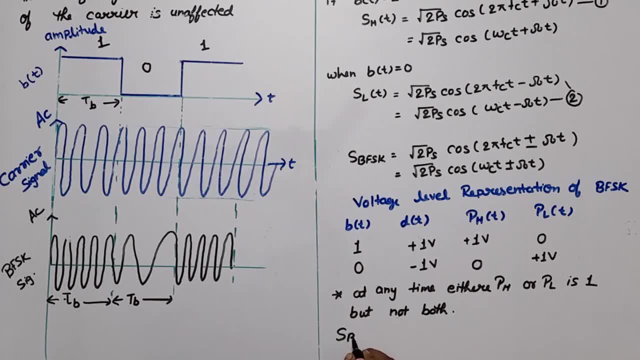 What can we write this equation: S B, F, S, K is equal to, under root, 2 PS, cos, 2, pi, FC. Okay, I will take T out. Plus minus means plus DT, ohm and T. Okay, The equation will be done for BPSK. 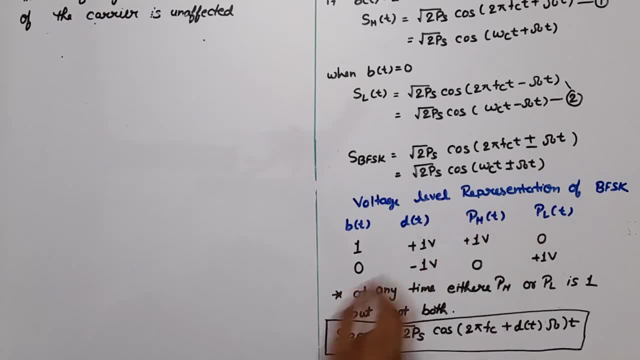 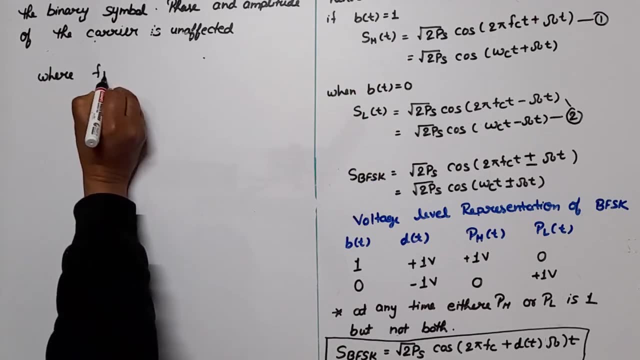 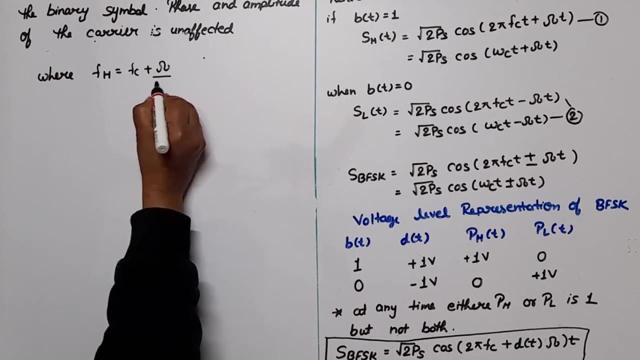 Now one more thing. From here you will be clear: PH and PL Are unipolar signal. If we see from this equation: High frequency FH is equal to What is it FC plus ohm? What will happen here? 2 pi. 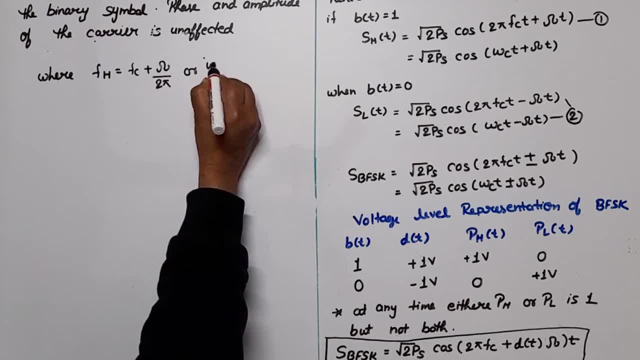 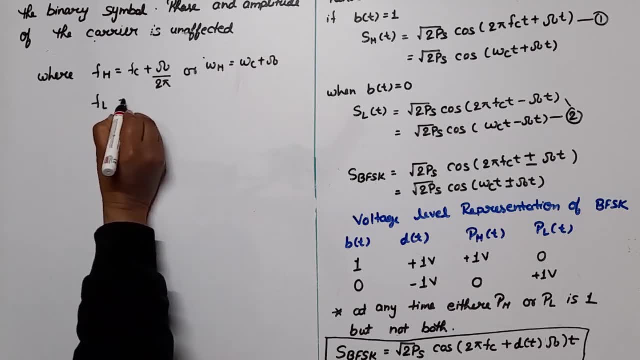 Okay, And what can we write this? Omega H is equal to omega C plus ohm. Okay, Same way. low frequency component FL is equal to FC minus ohm, 2 pi And Omega L is equal to omega C minus ohm. 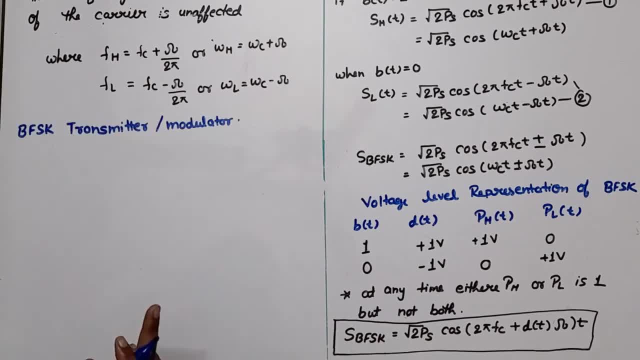 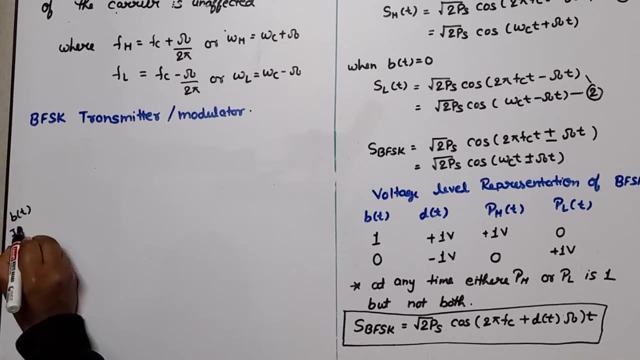 So basically what we will do here, We will do ASK modulation with two frequencies. In one case high frequency will be, In second case low frequency will be. Then we will add it Like this: What will happen first BT: This is input sequence. 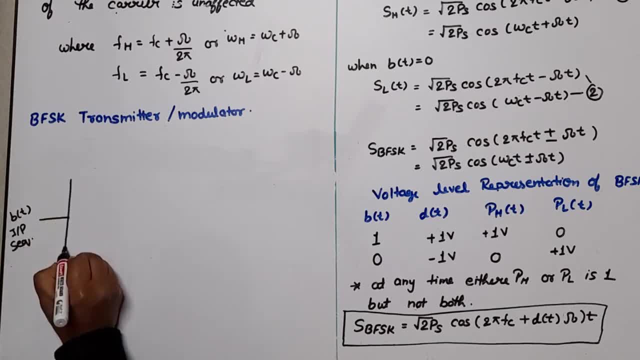 Clear. Now this is applied. Now we will have either 1 or 0. So we have two channels: One for our 1. And where our lower will be used. We will use inverter on this. This will be our opposite. 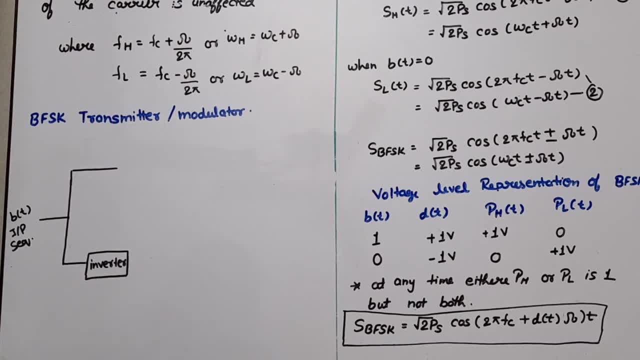 Okay, We need two channels, So we will direct on first And on second. we will give inverter. After that we will use label shifter In both path. Okay, Our label shifter will be here also, And then We will add. 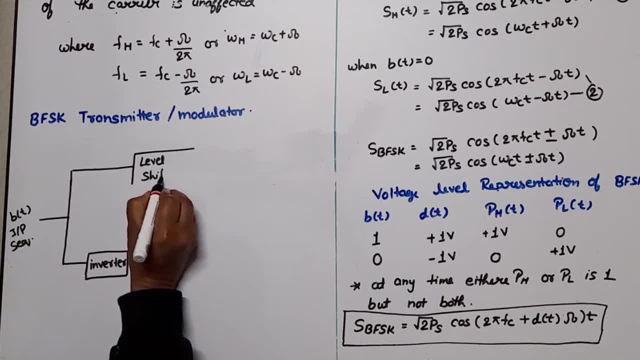 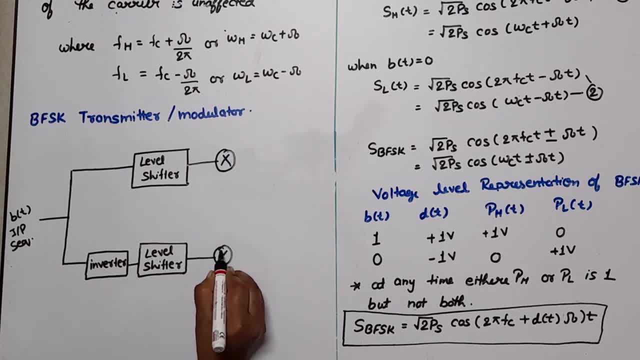 channels. Now what we have to remember is that for first, our frequency component will be high frequency and for second, our frequency component will be low. frequency component means here our phi1 is, that is under root, 2 by tb, cos, 2, pi, fht, and here our basis function is that 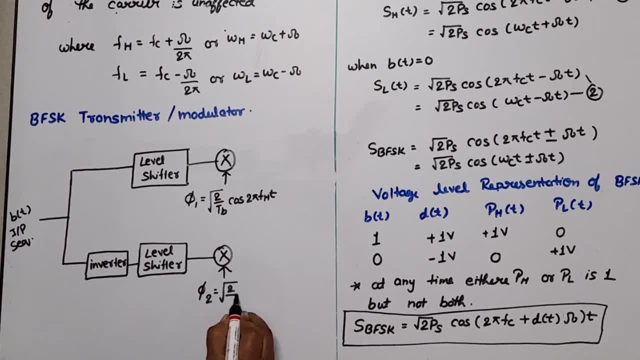 is. phi2 is equal to under root 2 by tb, cos 2, pi, flt done Now this output of product modulator we will give to both of them. we will apply on a summer. ok, We will put it here also, One side positive sign and other side also positive sign. 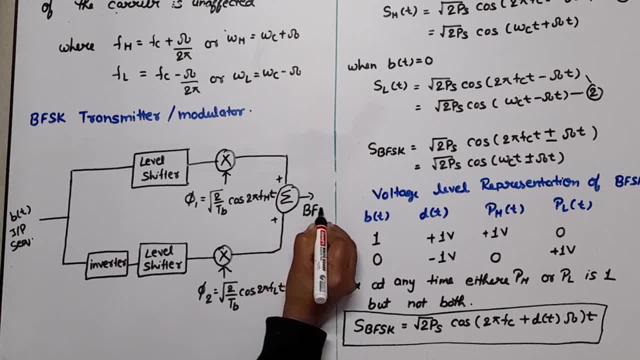 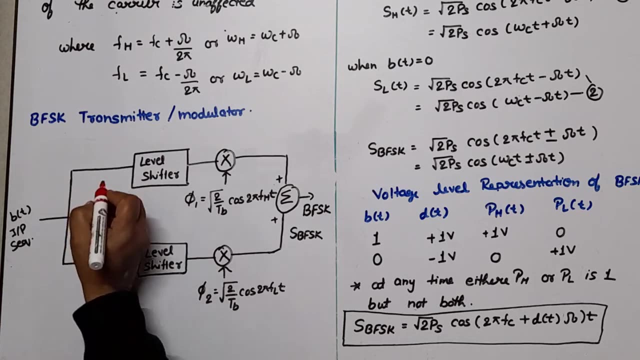 So, finally, what we will get here is signal that is bfsk, which is this one means sbfsk. ok, Now let us see its working. before that, we will put values also here, First of all when our inverter will be here. so here our signal will be pht, here our signal. 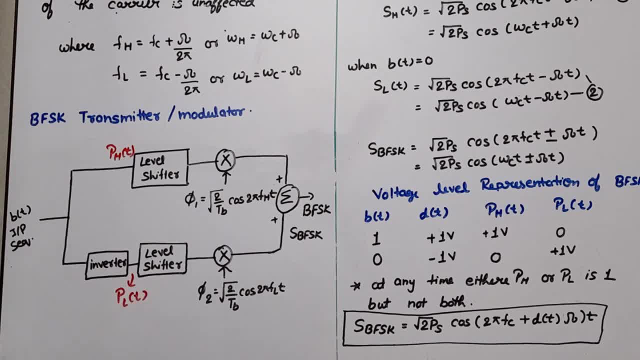 will be plt. ok. Then when our signal will be here, so here our signal will be plt. ok, So this signal is passing here. at this point it will be ps tb. this is the bit energy under multiplied with pht. ok, At this point it will be under root pstb, plt. now its working, suppose. now let us take an. 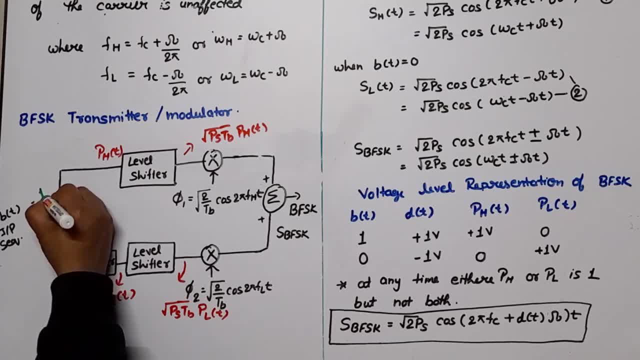 example, if bit is 1, ok, If it is 1, then by that number we will get this. So on this path our 1 will go. but here the 1 applied on input was 1 and what we will get on the output of inverter is 0.